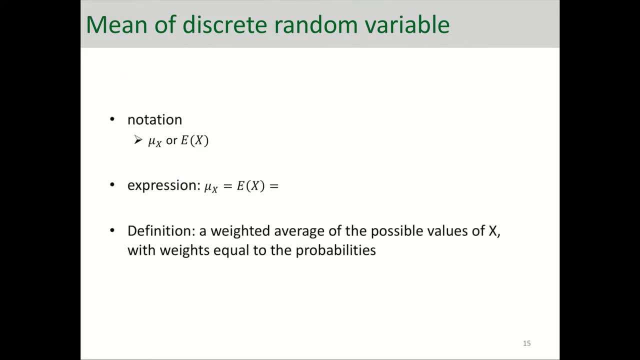 What's the notation for average or mean of a random variable? It is mu of x and x, representing the random variable, And mu represents mean or expected value of random variable x. So these are two common notations. Let's take a look at them one by one. 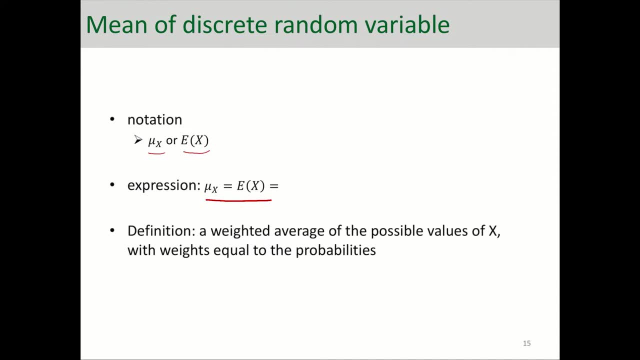 So we have two notations to use for average or expected value of a random variable And the way that we can calculate that is summation over values of the random variable on x, f of x. And you remember this f of x is the PMF function of random variable x. 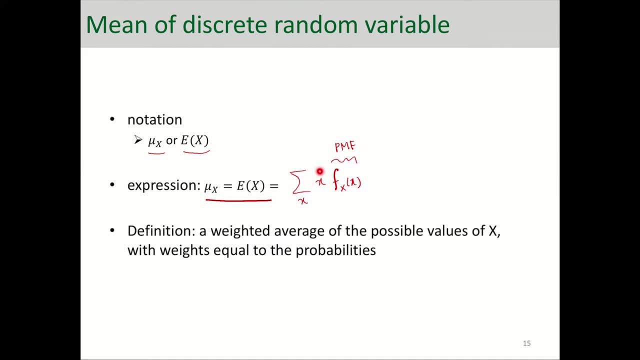 So we're essentially multiplying the values of the random variable x And we're multiplying the values of the random variable to the probabilities of those values. It is a weighted average, essentially of the possible values of x, With weights equal to the probabilities. 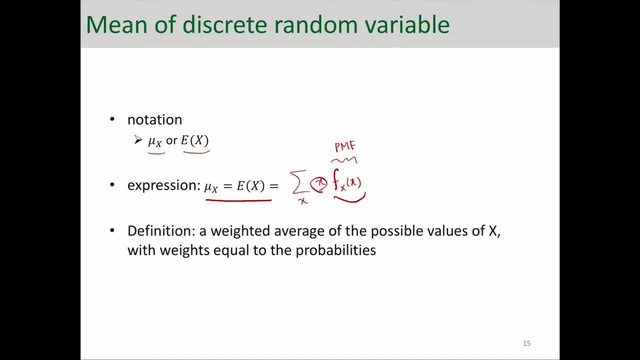 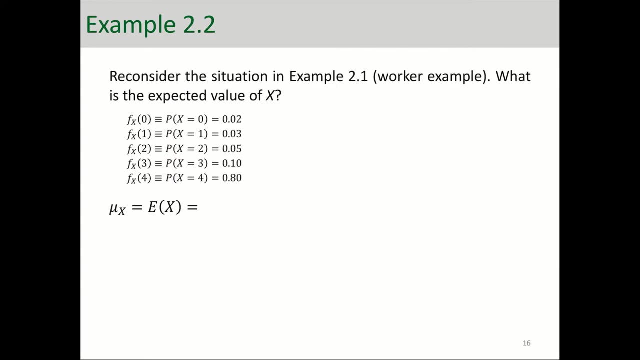 So here these are the weights And these are the values of x, And we're essentially doing a weighted average over them. So let's look at one example here to make this more clear. We're reconsidering the problem that we had before. 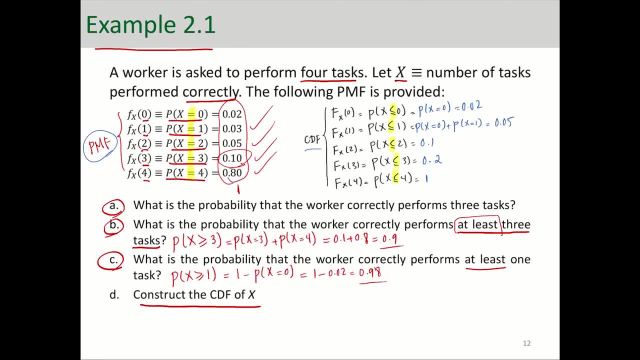 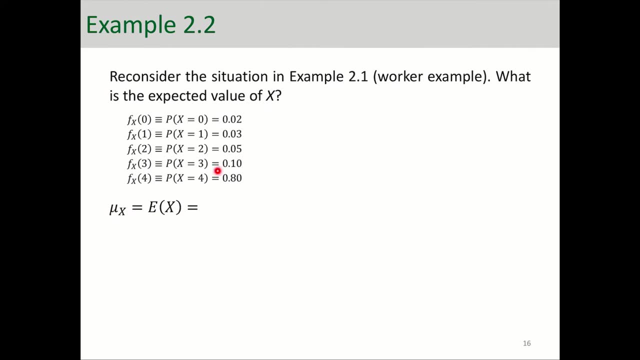 If you go a few slides back. this was the problem. A worker is asked to perform four tasks and x is the number of tasks performed correctly And the PMF function is given to us And the possible values of x is 0 through 4.. 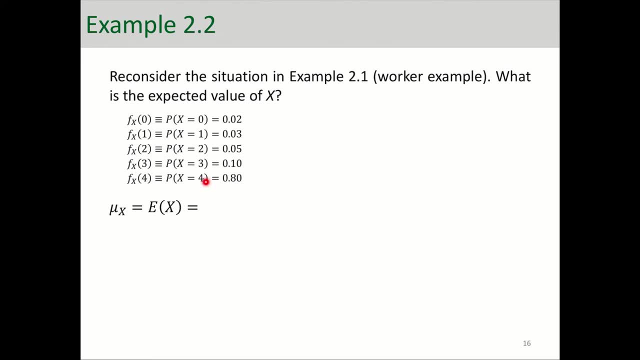 Either 0 tasks is being performed correctly all the way to 4. And we have the probabilities of them. So how do we calculate the expected value of this random variable? In other words, we want to calculate the average number of correct tasks performed correctly. 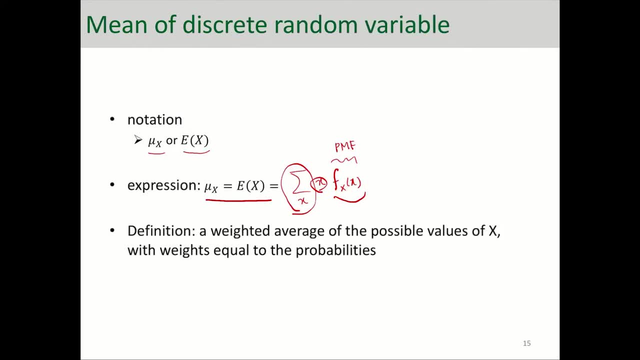 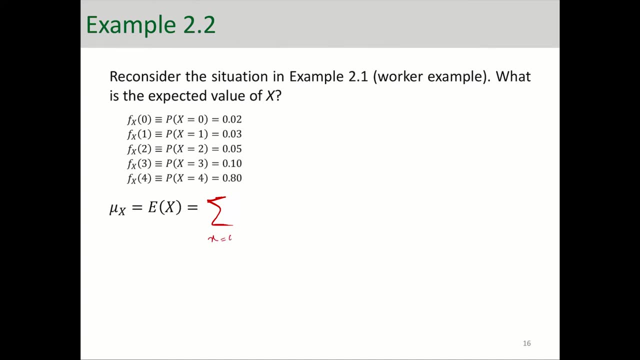 So, to follow the formula that we introduced here, that's going to be the summation over x values, And x values starts from 0 to 4.. x, f of x- The x values change from 0 to 4. And f of x values corresponding values are 0.02 all the way to 0.8..